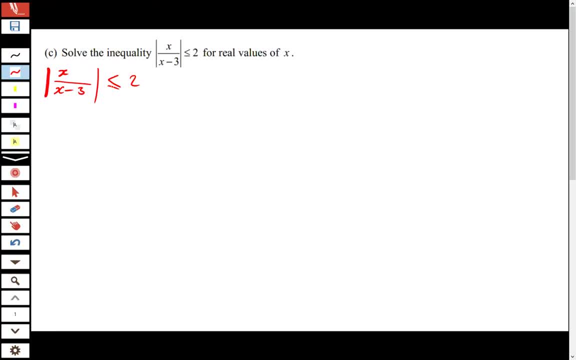 you have to take into consideration the rules that you have to follow when you're dealing with absolute value or absolute value or modulus value equations, Okay, Okay. so if you have anything which is in this format- let's say you have a absolute value of a is less than, let's say, you have k. So when you have such a question, this 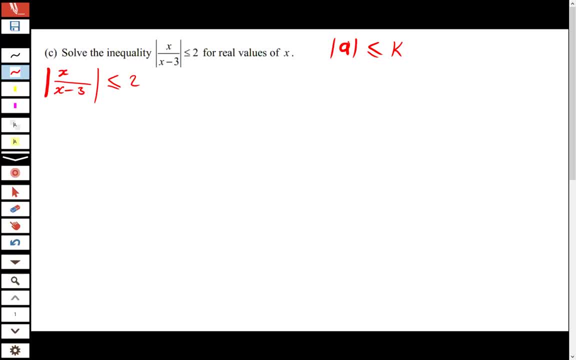 is supposed to be written, because we're not to say this absolute value, rather this a. the absolute value symbols can either be a negative or a positive number, because we're not to say the absolute value of a Is equal to a And even the absolute value of negative a will still be equal to a. So 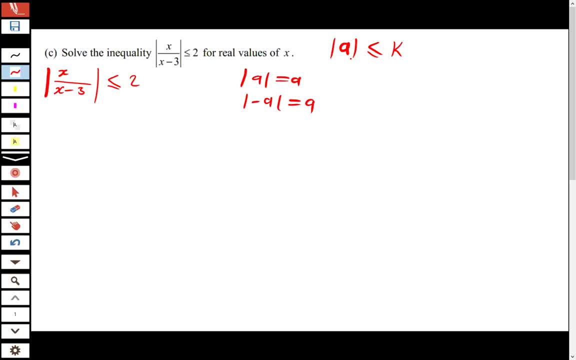 meaning what is inside the absolute value symbols here can either be negative or positive. So what that means is that we're going to say: the first equation that we're going to have is going to be a, which is a positive. a is less than k. And then we're also going 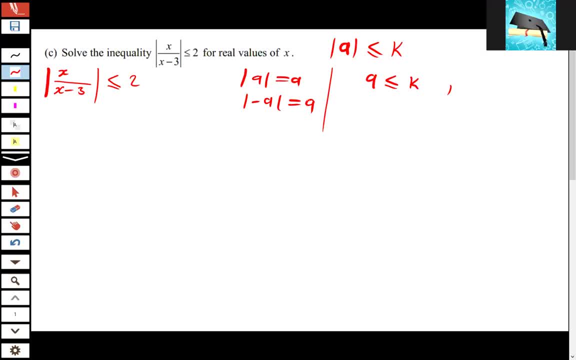 to have the second equation, which is going to be for the negative a. So how do you write that We say negative a is also less or equal to k. Then you solve these two equations separately to find the solutions. So this is exactly what we're going to do with this. 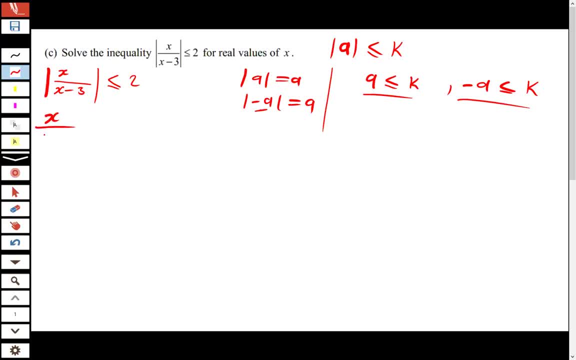 equation as well. So we're going to say: x over x minus three is less or equal to two. We also have the second equation, which is going to take the negative form of what is under the absolute value, which is, which is just going to be negative, x over x minus. 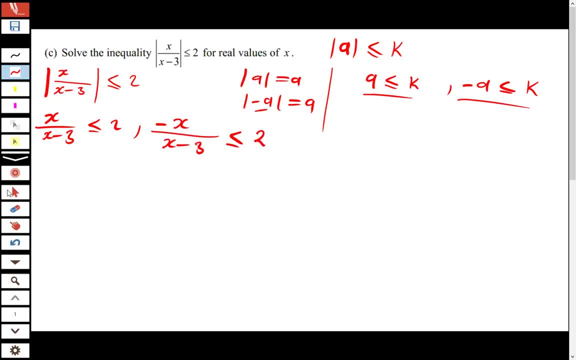 three, We say less or equal to two. So let's now solve the two equations separately. So I'll take the first equation, which is this one here. So for the first equation, like I said, when you have, when you're dealing with inequalities, in most cases, when you cross, multiply you. 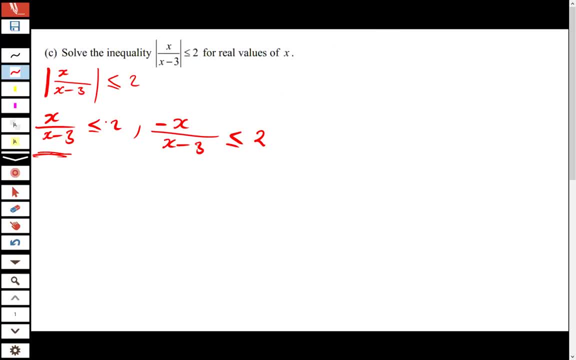 might end up getting a wrong answer. Sometimes, Yeah, So you might end up getting a wrong answer. So what you do is you take this number that you have on the right to the left side. Now what is x? So I'm going. 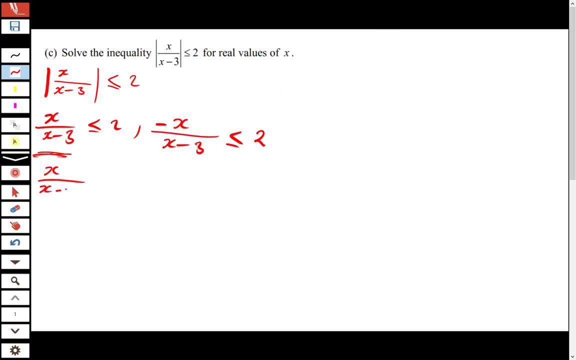 to have x over x minus three. and then we say negative, two less or equal to zero, Yeah, So now let us solve this equation. So we, uh, we express this as a single fraction By finding the common denominator this side. So the common denominator will be x minus three, because 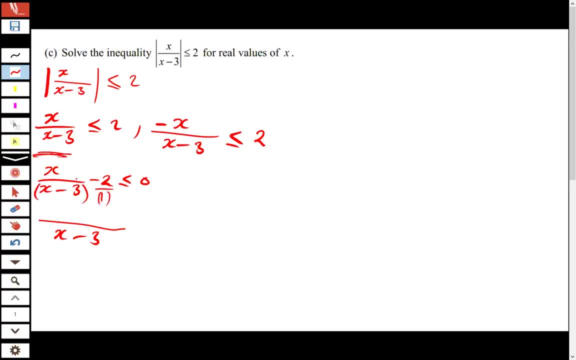 we have this part and then we also have one. So the common denominator, uh, where both one and X minus three can go into, is simply just X minus three. so when you say X minus three into X minus three, the answer is one one times X, or getting x. then we'll say one. 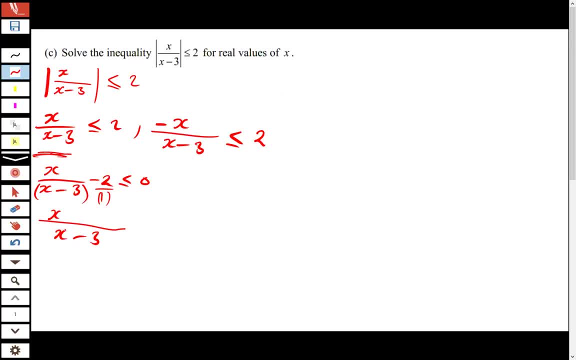 into X minus three. The answer is X minus three. X minus three times at greater than x minus three over one. Okay, How do we get X minus three? A remains zero at. the answer is zero minus three. negative two, which is just the numerator. there is going to give us negative two and then open. 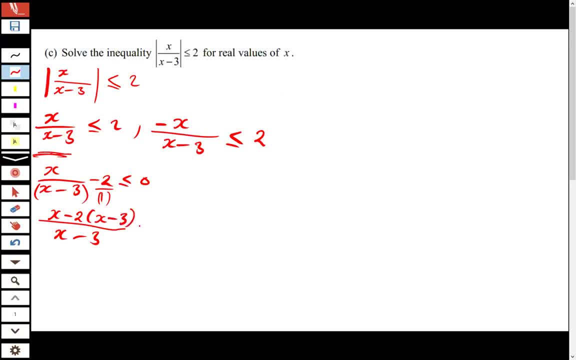 brackets, multiplying it with x minus three. you know saying this is less or equal to zero. Okay, so now we can simplify this on top, we're going to have x, then negative two times x. we're going to have negative two x, And then the other thing is negative two times negative three. 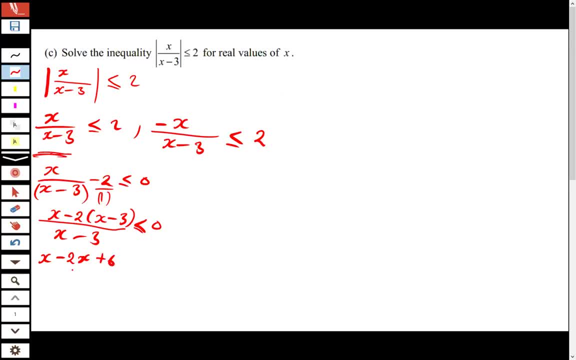 we're getting positive six, then everything down here. we're going to have x minus three and say less or equal to zero. So when you add the first two terms here- since they're like terms- we have x and negative two. when you add them you're going to get negative x and then plus six. 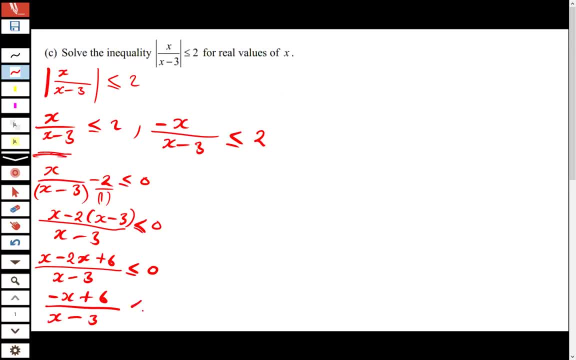 everything divided by x minus three, then this will be less or equal to zero. So now, when you reach here, you now have to get the critical points And then you put them on the number line to test them, to see which region qualifies for this expression. So how do you do that? So let me just demarcate. 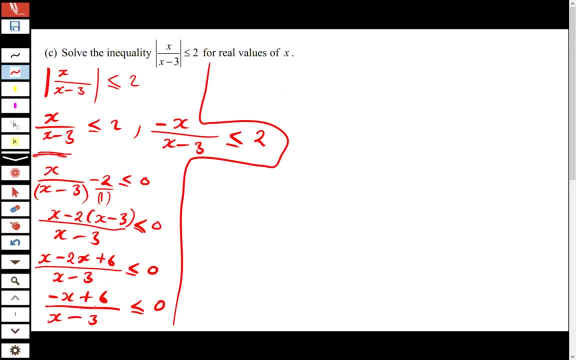 So I'm going to equate the numerator- both the numerator and the denominator- to zero. So when I get the numerator, I'm going to have negative x plus six is equal to zero. Then when I simplify this expression, I'm going to have negative x is equal to negative six When I divide everything. 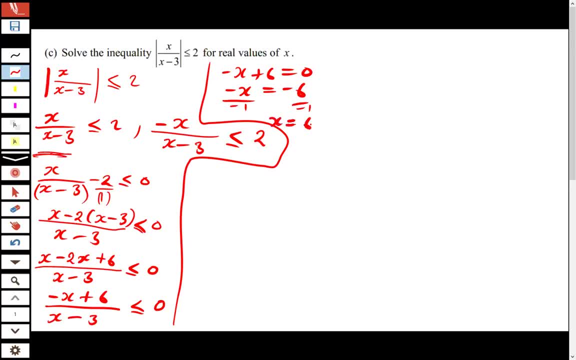 by negative one, I'm going to get x is equal to six. Then I'll also do the same for the denominator, where we have x minus three and we put this to zero. So when you get that to zero, we're going to get x is equal to positive three. So these two values are the ones that we're. 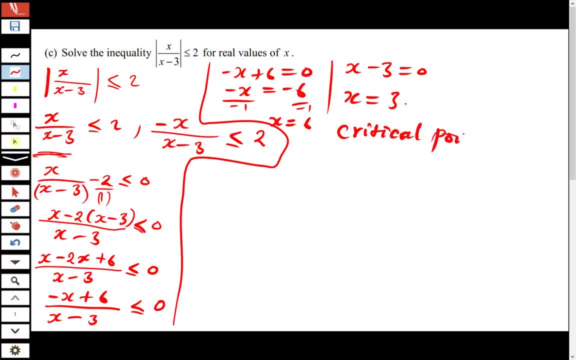 calling the critical points. So these are not the final solutions, These are just critical points. Now we're going to use these same two critical points to find. we're going to use these two critical points to now determine the region which is going to make this statement that we have here to be true. So how are we going? 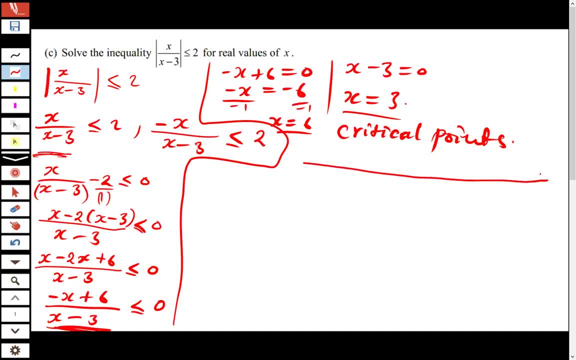 to do that. I'm going to draw a simple number line here And I'm going to put my critical points there. So on the critical points we have, I'm going to put my critical points there. So on the critical points, we have three. then we also have positive six. So this side, we know that. 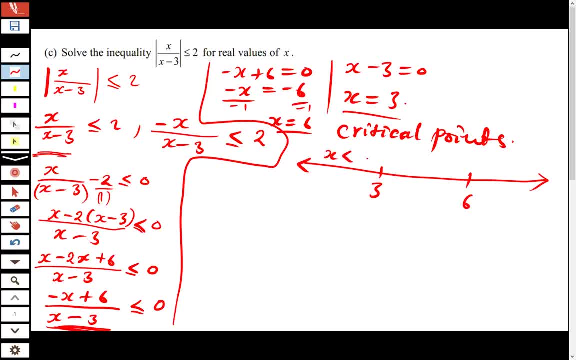 these are numbers that are these x values. this side are less than three. So now, because we're using less or equal to three, we're going- I mean, since we're using less or equal to symbol in this expression, we're also going to be putting less or equal to that, And then numbers between: 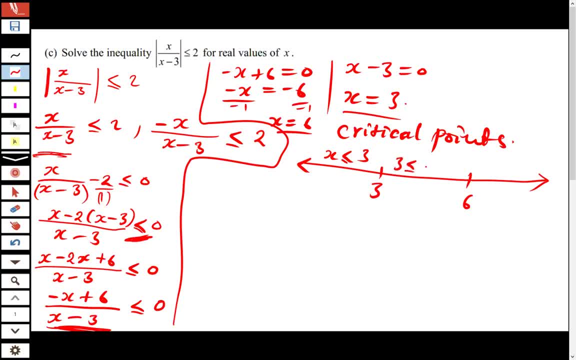 three and six. we write them as three less or equal to x less or equal to six, then numbers greater than six, all the numbers that are this side. So these numbers are the ones that were saying. So these numbers are the ones that were. 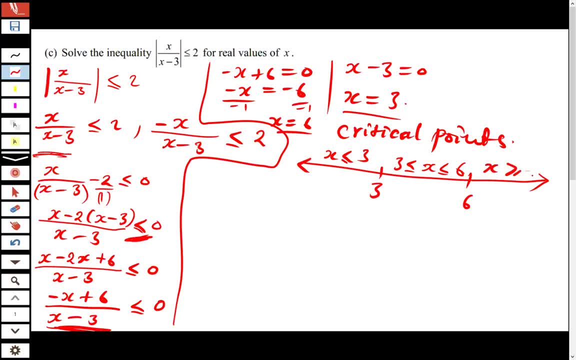 going to say x is greater or equal to six. So now we can start testing the regions. So how do we test the regions? So, numbers that are less or equal to three, we can get any number that is less or equal to three. Okay, let's, let's, for now, let's avoid. 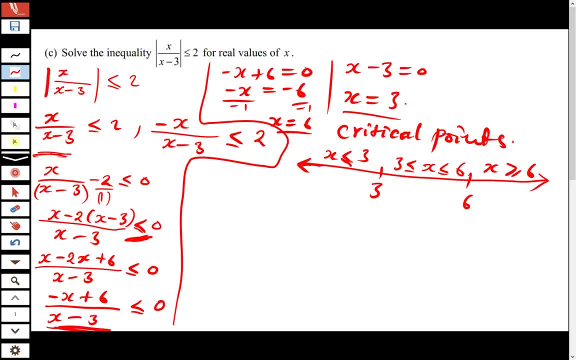 three. let's just get any number that is less than three, And I think we can get to. I think let's just use zero so that we don't waste time thinking about how to calculate. So if we put zero x in this expression, so let me just copy this same expression here. So we have negative x plus. 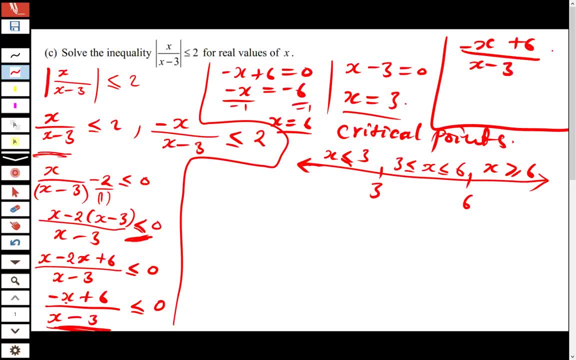 x minus three, then we say this is less or equal to zero. So if we put zero, because zero is less than three, so if we put zero at x there, so if I put zero, what is x here? I'm going to have zero plus six, which is going to give me positive six. So I'm just 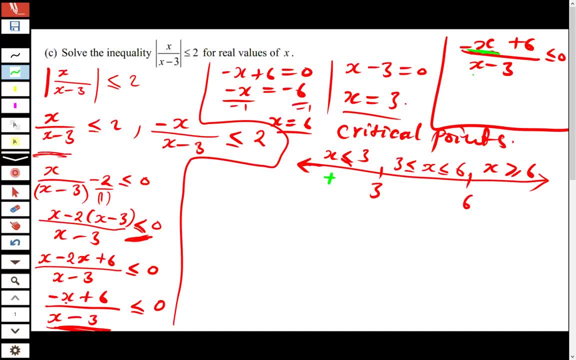 going to write a positive And then, if I put zero positive six, I can also write a positive where there's x. there I'm going to have 0 minus 3, which is going to give me negative 3.. So I'm. 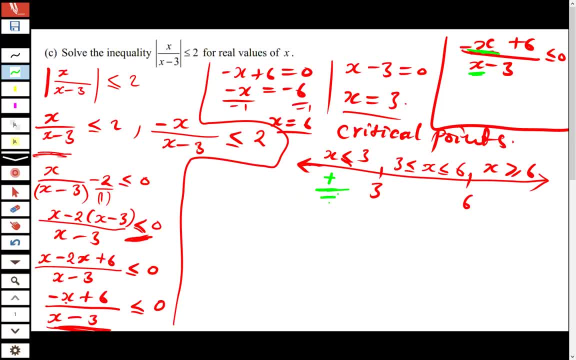 just going to write negative as the denominator. So we have positive divided by negative. So positive divided by negative, the answer that I'm going to get is going to be a negative. So when you divide a positive number and a negative number, the answer that you get 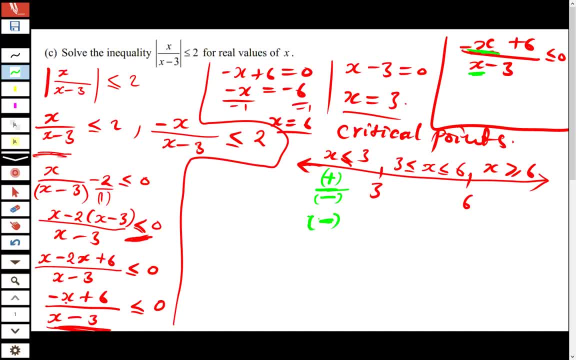 will be a negative number. So now you have to ask yourself one question: Is a negative number less than, following this symbol here, is a negative number less than or equal to 0?? The answer is yes, which implies that this is one of the regions that we're looking for. 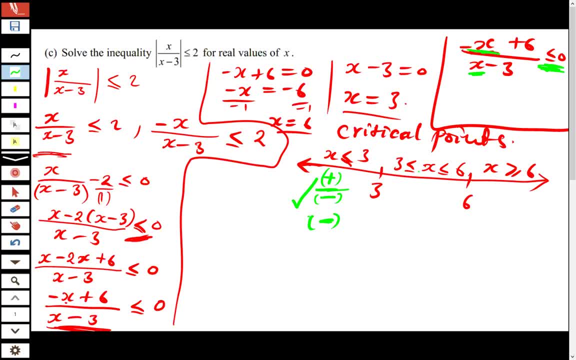 Let us try to test the region between 3 and 6.. So we get any number that is between 3 and 6. We can even get 4 or 5.. So if I get 4 and put it where there's x in this expression, 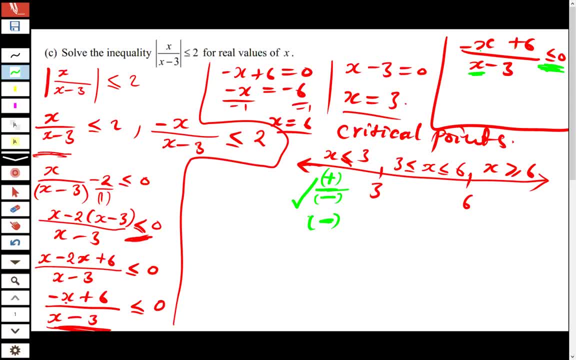 I'm going to have negative 4. Plus 6. So negative 4 plus 6 will give me. so negative 4 plus 6 is going to give me positive 2.. So positive 2, I'm not going to write positive 2.. I'll just write positive there. 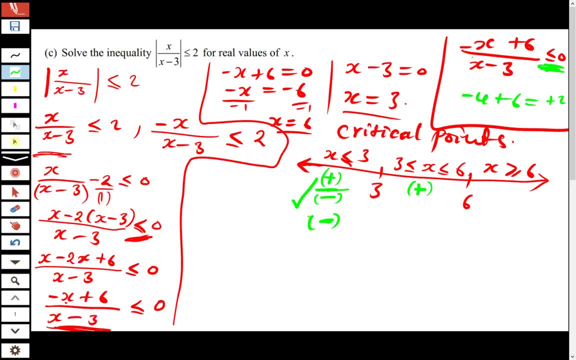 So I'll also do the same on the denominator. I'm going to replace x with 4.. So if I put 4, I'm using 4, because I know that 4 is between 3 and 6.. So if I put 4,, I'm going to get 4.. So I'm going to get 4.. So if I put 4,, I'm going to get 4.. 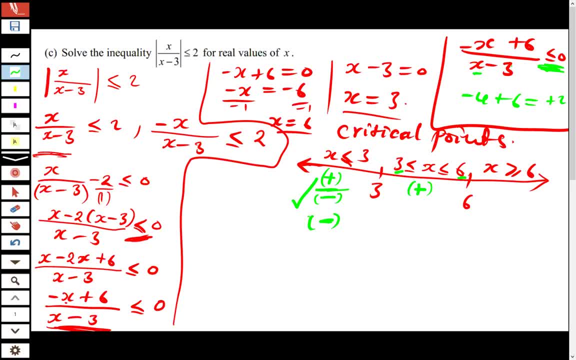 So if I put 4, there's x there, I'm going to have 4 minus 3.. So 4 minus 3, the answer will be a positive answer. So I'm going to put a positive as the denominator. So positive divided by positive, the answer will be positive. 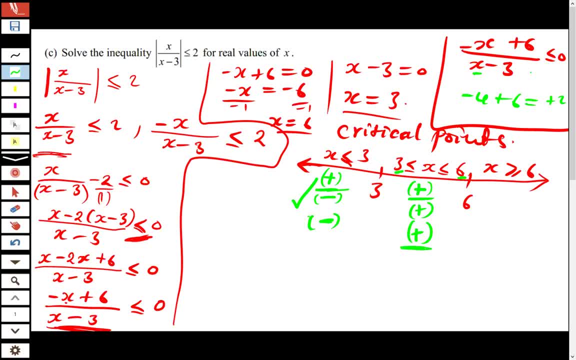 So now, is a positive number less than 0?? If it's a positive number less than 0, the answer is no. Hence this region is going. this region is rejected because when we get any number between three and six, the answer that we're getting is positive. 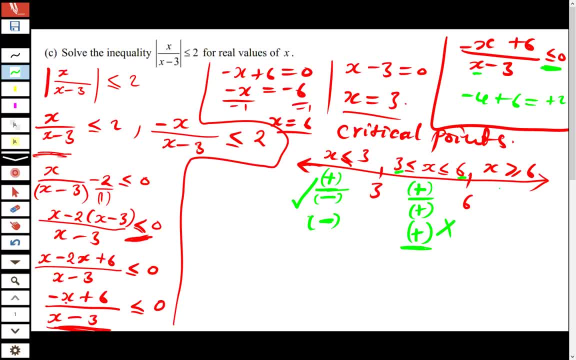 which is not making this statement true. So let us test any number that is greater than six. So we test any number that is greater than six, We can even get seven. So when we put seven, there's X here. We're going to have negative seven plus six. So negative seven, negative seven. 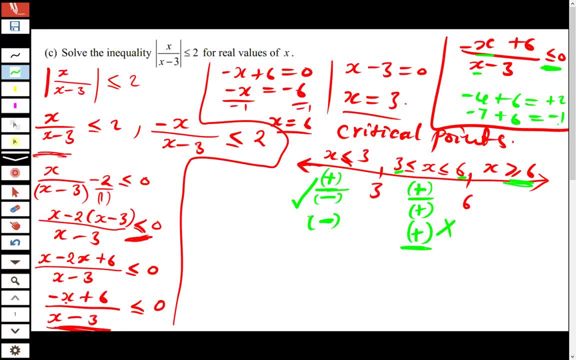 plus six, the answer will be negative one. So negative. seven plus six, the answer will be negative one. So I'm just going to put a negative there, Then I'll say over. And then we also put seven there. So I'm going to have 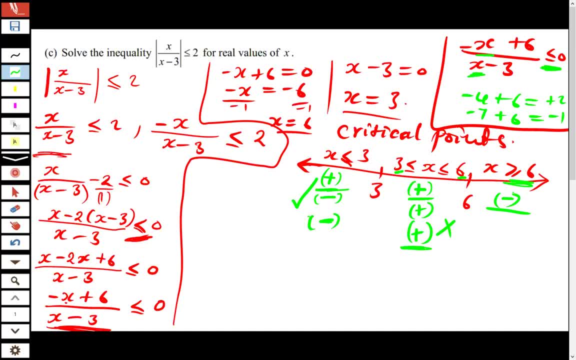 seven minus three. So seven minus three, the answer will be positive four. So I'm just going to write a positive there. So negative divided by positive, the answer will still be negative. So is a negative number Less than zero? The answer is yes. So this region is also making this statement to be true. 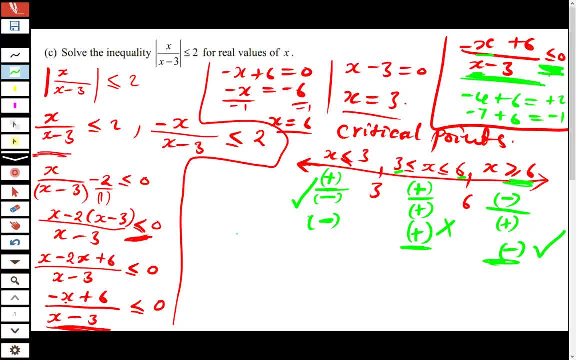 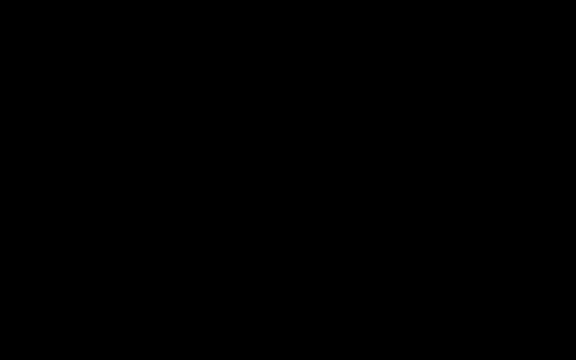 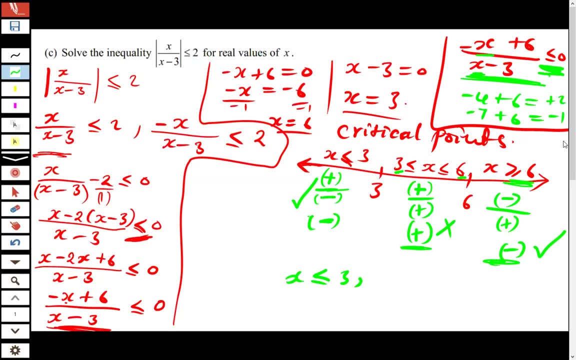 So the region or the range of values of X that we're looking for. So the region that we're looking for is simply just X. So X is We're looking for this region, X is less than three And also X is greater or equal to six. 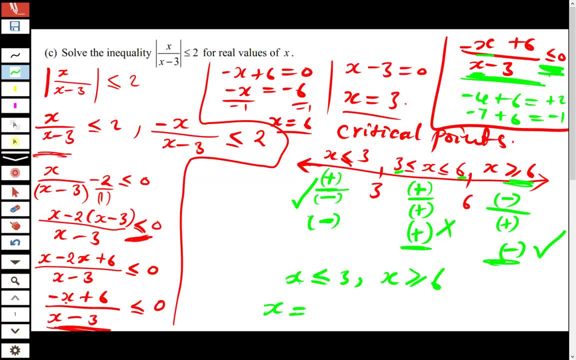 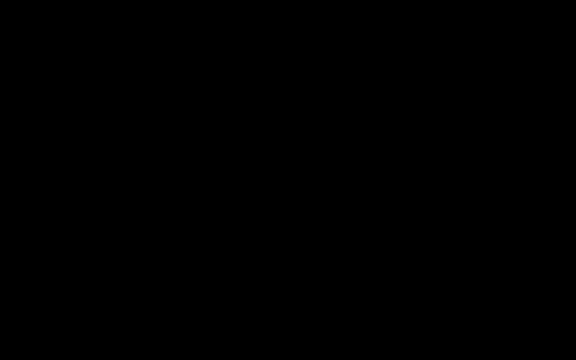 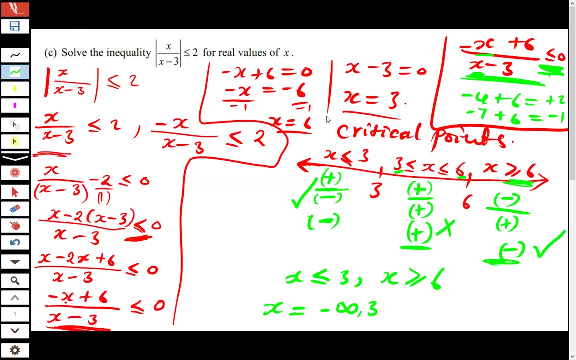 So, if you want, you can write it as: X is equal to. We know that numbers that are less than three are just ranging from negative infinity. Okay, so I was saying so. I was saying so. this expression here can also be written as: x is equal to negative infinity up to three. 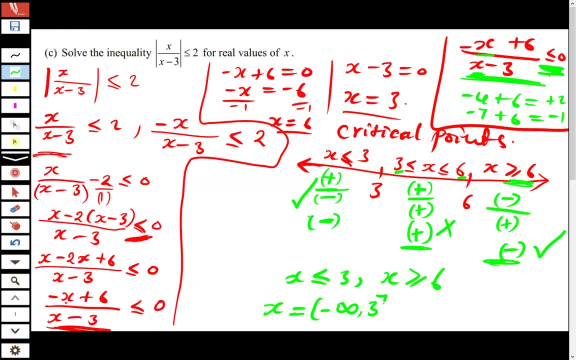 But because we're saying less or equal to three, meaning we're going to use a closed bracket at three, then we say union, we are again starting from six up to positive infinity. So you can either write it like this or like that. 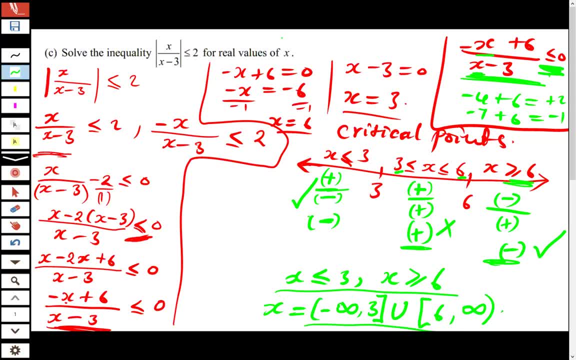 The answer is to you the same. They both mean the same thing. OK, So this is exactly what you're supposed to do. Do you have any questions before we solve the next equation? So we'll solve this one. We are not supposed to solve this other one here. 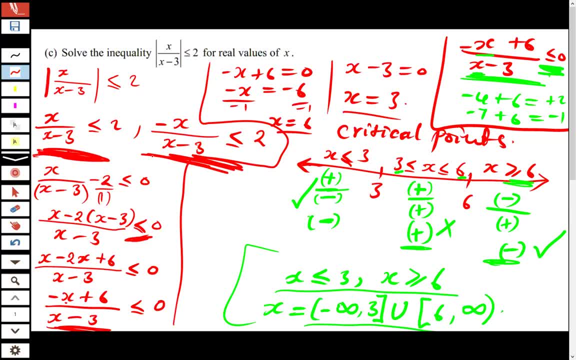 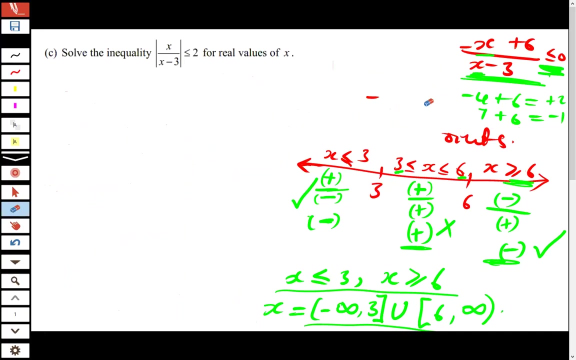 Do we have any questions on the first equation? OK, so let's proceed. No, OK, So we took the positive part. We're now going to take the negative part of that equation. OK, OK, OK, OK, OK. 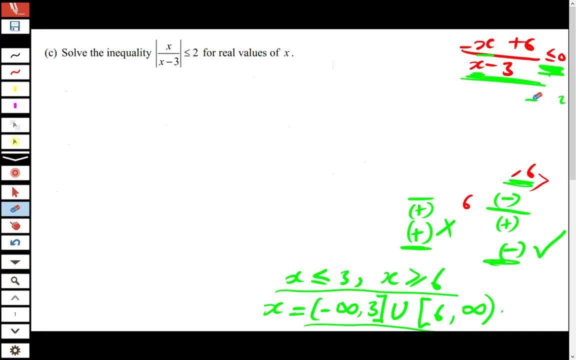 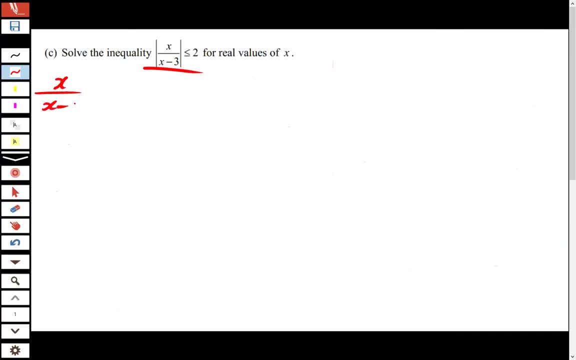 Remember what I said. I said this expression can be written as X over X minus three less or equal to two, x over X, and also x negative, x over x minus x minus three less or equal to two less or equal to two. So we've solved this one. 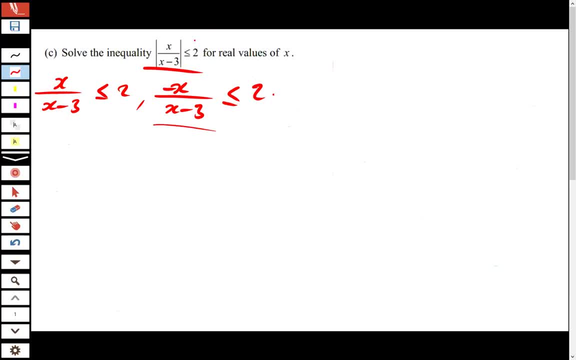 We now have to solve. We now have to solve this one. So for the first one we got the answers to be: X is equal to negative infinity comma three. This is the for this equation here. we got this as our answer, And then 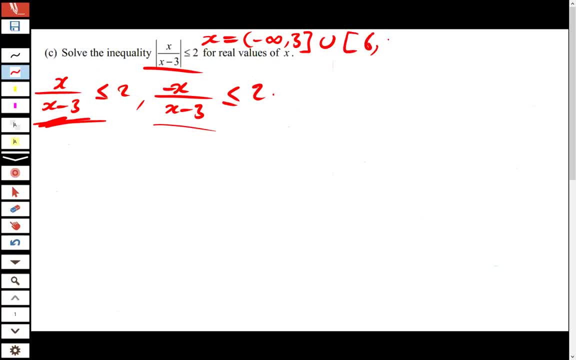 we say: union um six comma positive infinity. This is what we got. Now let us solve this one. So something, this one, we're also going to do the same. We take this two on the right, we take it to the left, So I'm going to have negative X over X minus three. Then we say: 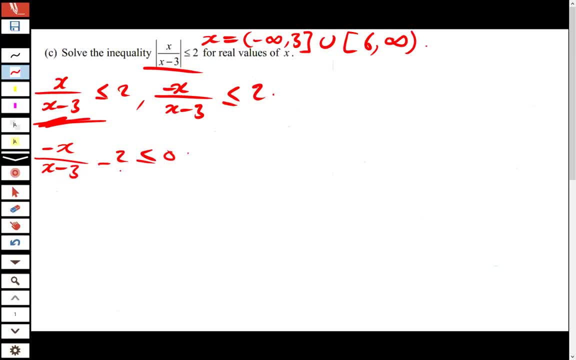 minus two is less or equal to zero. And then we find the common denominator, which is just X minus three. Then from there we're going to say X minus three into X minus three. The answer is: one, one times negative X, we're getting negative X, Then one, two, X minus. 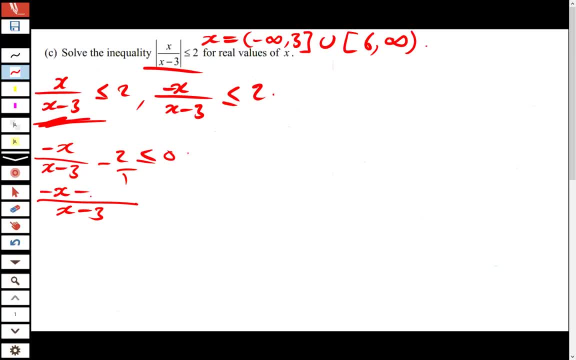 three. we're getting X minus three times negative two. We'll have negative two multiplying X minus three. Then this side, you have less or equal to zero. So we get negative X minus three. And then we have negative two times negative three. So we get negative X minus. 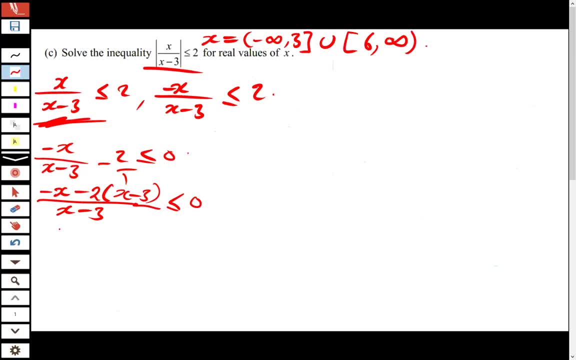 three equal to zero. Then we can simplify the numerator there, So the denominator is two X minus three. Then the numerator will be negative X, then negative two times X, We'll get negative two X. negative two times negative three, We're getting positive six. 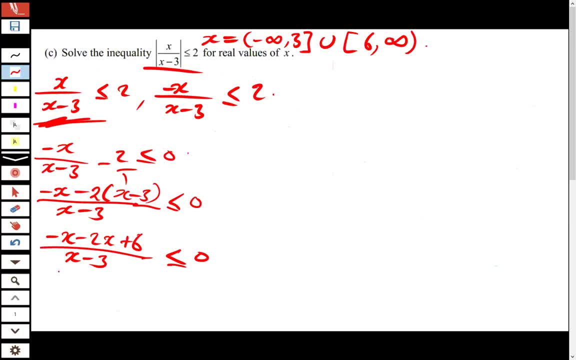 Then this is less or equal to zero. So when you simplify this expression, we're going to have um negative three X plus six over zero. Okay, We say less or equal to zero. So to find the critical points, we're going to equate. 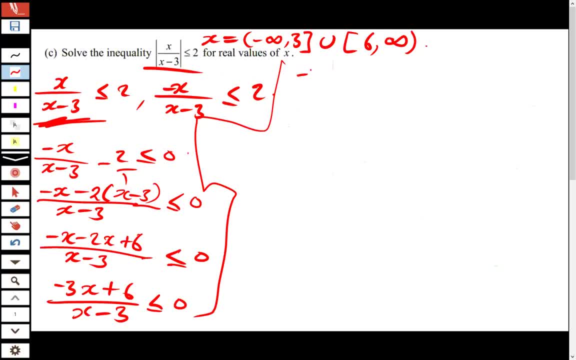 both the numerator and the denominator to zero. So we're going to have negative three X plus six is equal to zero. And also we'll have X minus three is equal to zero. So when we simplify this expression, we're going to get negative three X is equal to negative. 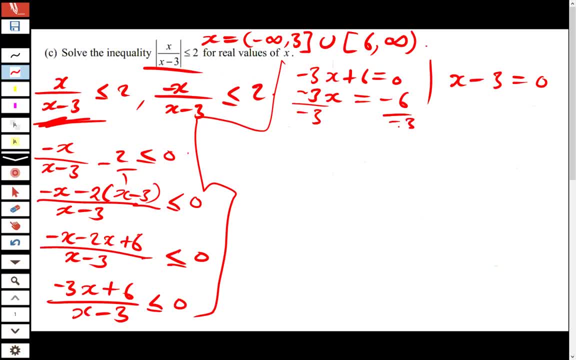 six. When you divide both sides by negative three. negative three, or getting X is equal to a positive six, uh, rather, positive two. And then this other side I just want to have, X is equal to positive three. So, after finding these two critical points, can now take them. 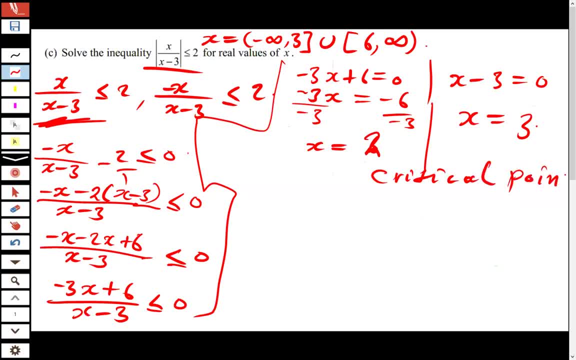 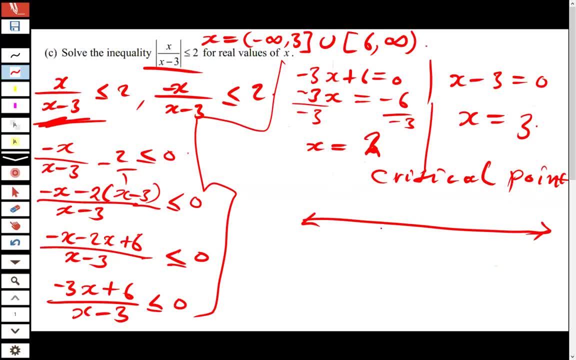 that we can find the correct region which we're looking for. So I'm going to put- I'm going to put two there, Now also put three. So I know that all the all the numbers, that this side they are less than two. So I'm going to say: this side we have X less, or 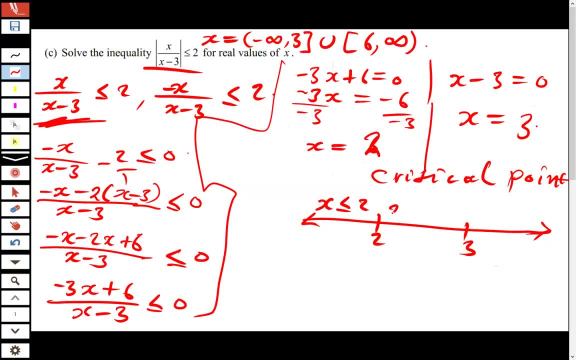 equal to two. Then here in between two and three, we have numbers that are between two and three and we can write in, we can, we can write it down, we can write this: regionals what you're seeing here, what I've written: two less or equal to. 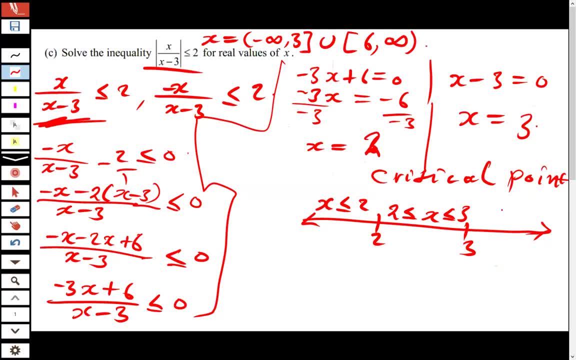 x, which is less or equal to three. the numbers that are this side are numbers that are greater than three. okay, so now let's take any number that is less than two. then we test it in this expression here. so when I get lesser, for instance zero, because I know that zero is less than two. so 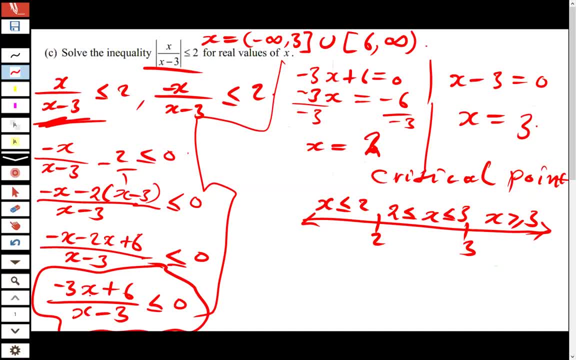 I can use zero. so when I put zero as x there on top, I'm going to have zero, because I know that negative three times zero, the answer is zero. so zero plus six, the answer will still be positive six. so I'm just going to write a positive there and then, if I put a zero over this x here, I'm 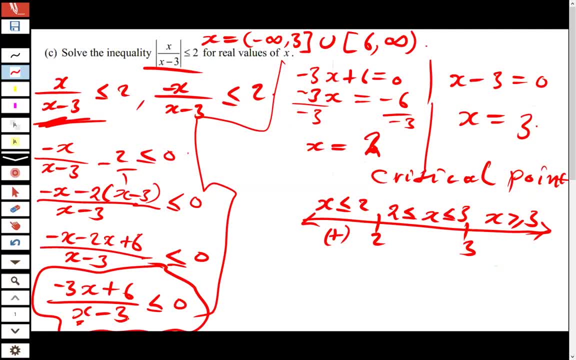 going to have zero minus three, which will give me a negative. so now the equation comes in to say: or, before we ask ourselves that question, we can say: we can first simplify this positive divide by negative. the answer is negative. now is a negative number less or equal to zero. 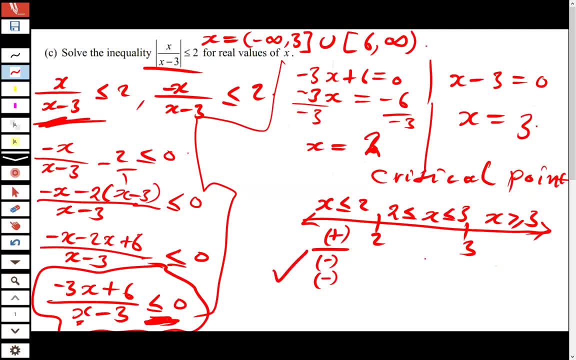 the answer is yes, so meaning this region is also as accepted. so let us also test any number that is between two and three, so we can even get 2.5. so when you put 2.5 where there is x, there we're going to have. 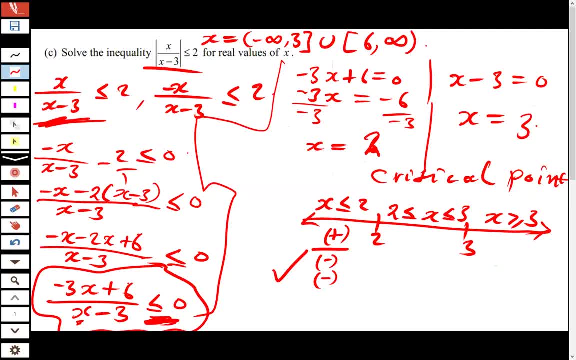 2.5 times three, and then we add it to six. so two, two point five times three, then we add it to six. we know that two times three gives us six. so if we say two point five times negative three, the answer will be negative, something like negative seven, yeah, which is. 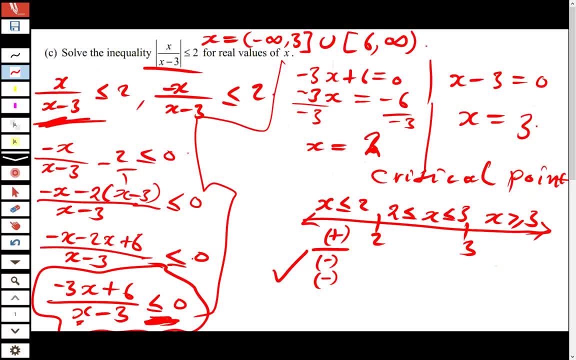 I mean which when added to six. but we're still going to get a negative answer. so when you simplify, when you put 2.5 where there's x and then we add it to six, the answer that you're going to get will be a negative then denominator there: when. 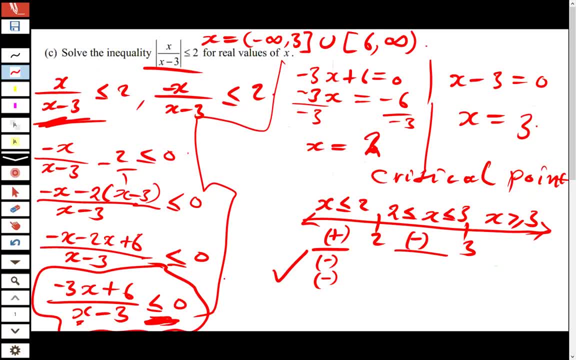 you put 2.5 there. we say 2.5 minus 3. the answer will be a negative. so negative: divide by negative. the answer is positive. is a positive number less than zero? the answer is no. so this region will be rejected. we can get any number that is greater than three. so 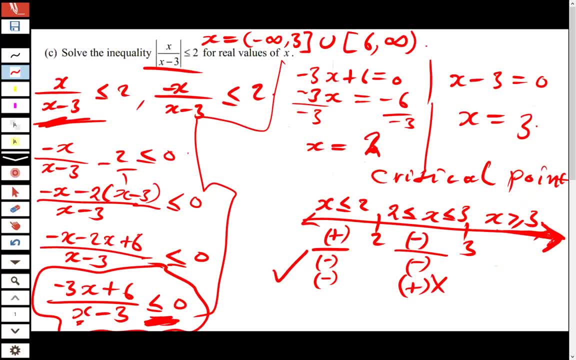 that we test for this other region so we can get four. when you put four where there's x there, we're going to have negative. I mean negative three times four, to give us negative twelve. negative twelve plus six, the answer will be negative six. so just I'm just going to write a negative there. 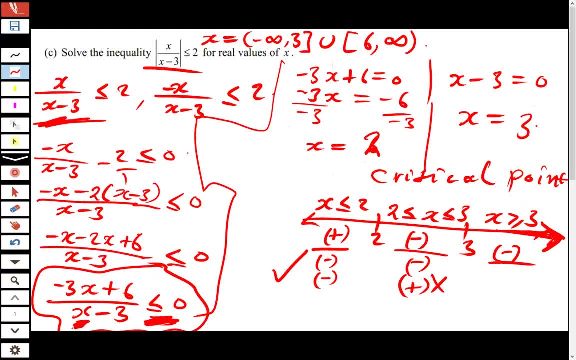 and then when I put a negative 12 y, this, or rather negative, not negative. when I put four, this x there because I'm taking numbers that are greater than three. So when I put forward is X, I'm going to have four minus three, which will be a positive one. 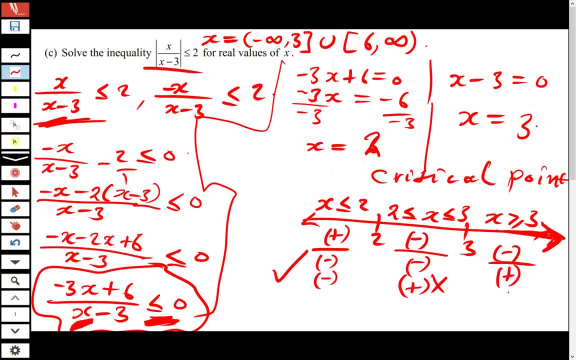 So I'm just going to have a positive there. So negative divided by positive, the answer will be negative. So is a negative number less than the negative number less than zero? The answer is yes. So these two regions are the ones that are accepted. So now we have 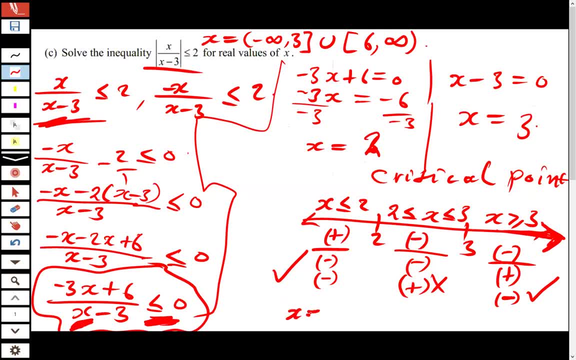 the range of values of X. for the second equation to be: X is equal to numbers that are less than two. can also be written as numbers ranging from negative infinity up to two. And then we are. we're finding the union set, which is union. In other words, it's just the addition of two. 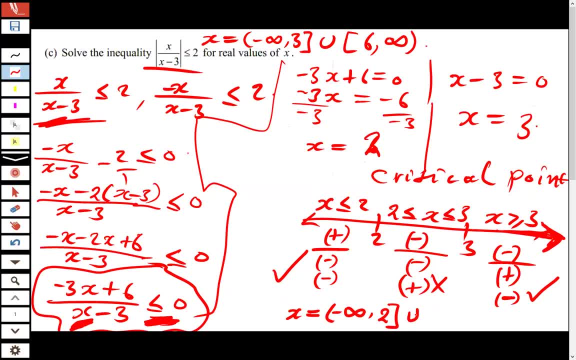 different sets. Okay, So we're finding the union set of this and also the numbers that are greater than three. So many are going to have three there, up to positive infinity. So now to find the final solution, which is um, the, the, the, the set of values that are going to make this. 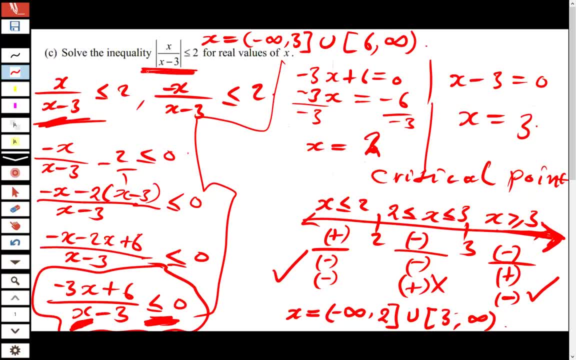 um, th, th, th. this equation true, we are going to add or we're going to find the intersection set of this expression here and what we have found there. So when we find the intersection set between the two expressions, then that's the solution set, for that's the 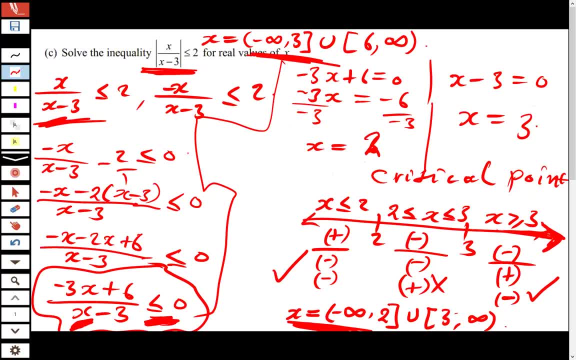 solution set, which is just the final answer that we're looking for. So let us find the intersection. I'm going to use a blue color, Okay? So I'm going to name my first X as X one. So let me say: this is X one, Then this one is X two. So to find the final solution. 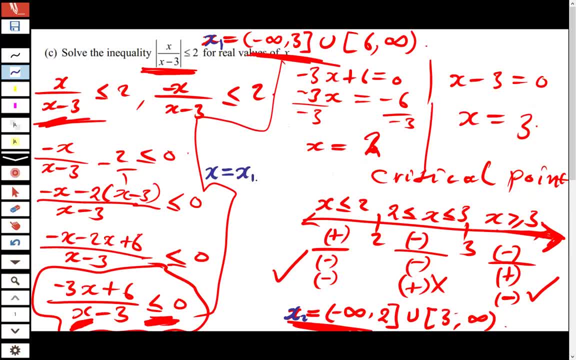 which is just X. we're going to say X is equal to X one intersection X two. So X one intersection X two. I'm going to find the intersection set between the first X and the second X, So my value of X therefore be equal to. 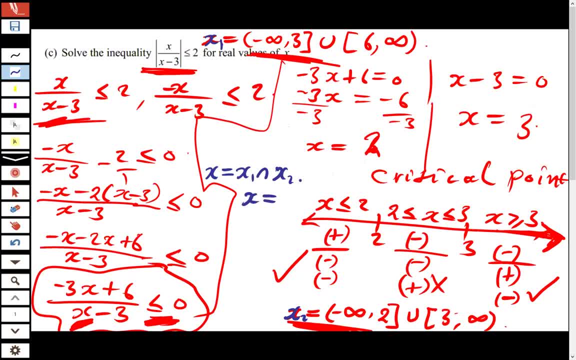 let me just erase this part, okay. So I'm going to simply understand this in the drawing. So the value of x or the solution set, is now just going to be- it's not just going to be- the intersection set between what we found there and what we found for the first. 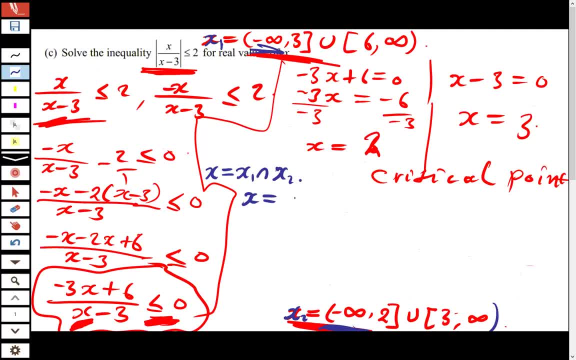 equation. Okay, so the intersection of these two equations will be will be from negative infinity. then we get the smallest number between the two sets in the, I mean in this first set, we get the smallest number. So in this first set the smallest number is two. we have two there. we also have three. 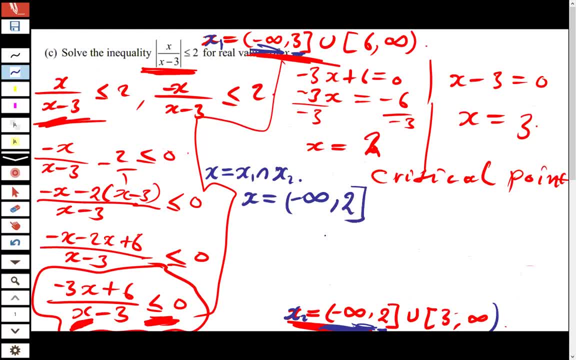 there. So I'm going to get to then our close, then I'm going to say union. then in the next set I'm going to look at the biggest number, want to look at the biggest number because we're looking for the intersection set. for if we're looking for the union set out of looked for, 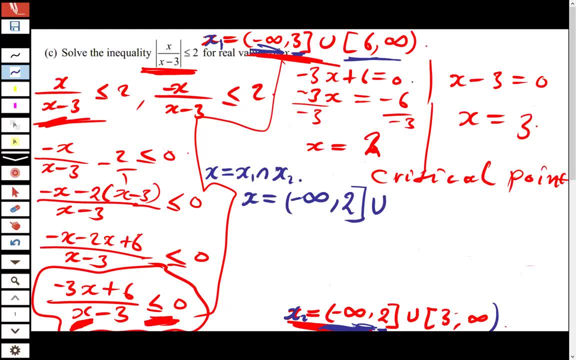 the smallest number, But in this case we're looking for the smallest number, Okay, Okay. So we're looking for the intersection mean, the common, the common elements. So I'm not going to get the smallest number, going to get the biggest number. 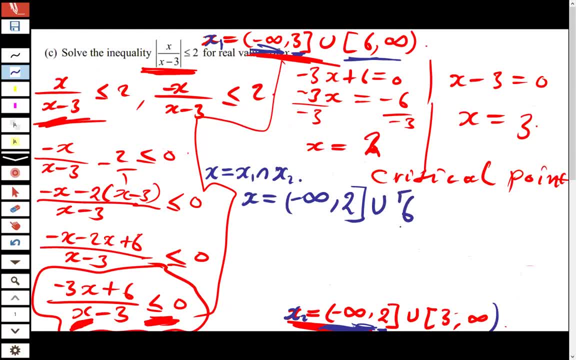 So in this case we have six there, So I'm going to put six there. then say: comma, positive infinity. So this is the solution set. So when you get any number starting from two going to the negative infinity, try to put: 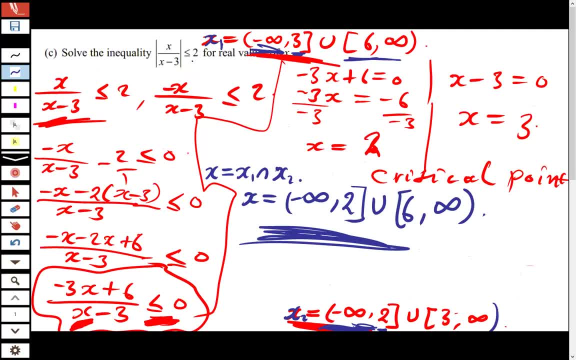 it in this expression, you discover that the answer that we're going to get to either be equal to two or to be less than two, Or if you get any number that is greater than or equal to six, the answer that you're going to get if you replace it in this expression, in this equation, you discover the answer. 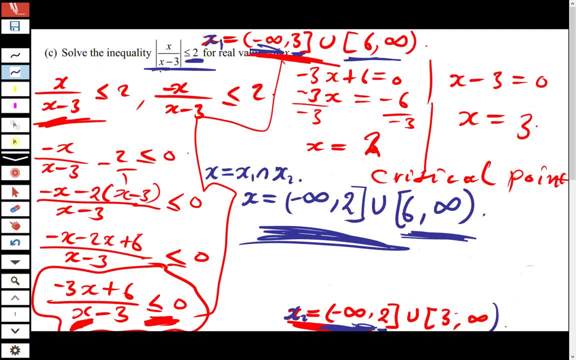 that you're going to get to be less or equal to two. So this is how you solve such inequalities. Okay, so the most important thing is just to come and find the intersection set between the two sets of two values, two sets of two values. 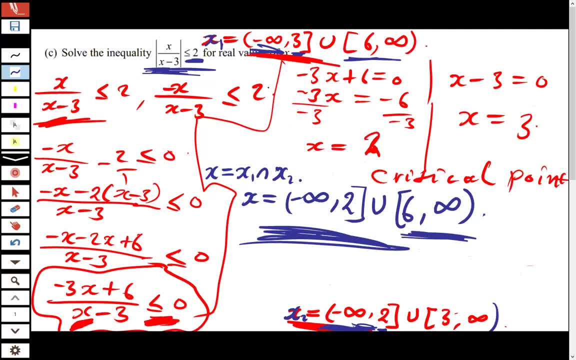 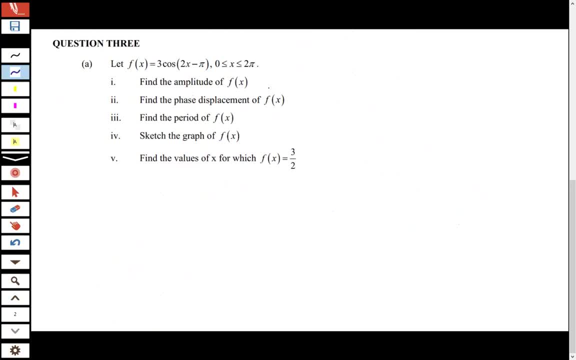 The values of x that you found. okay, let's look at question three. So this is question three in the assignment And then tomorrow- rather on Wednesday, we're going to proceed with the other questions. I'm sure on Wednesday we'll be done with this assignment. 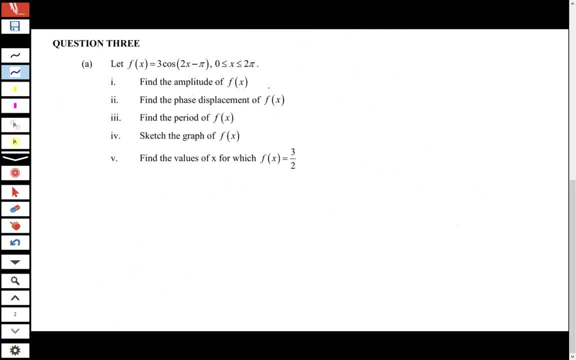 So that next- I mean so that on Friday we just begin a new assignment, which is assignment two. Okay, So for question three, this is also straightforward, Okay. so I think let's do this. You can just join using the same link. let me just change the time because it's showing. 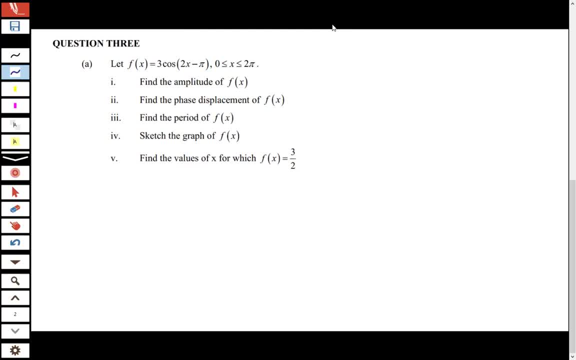